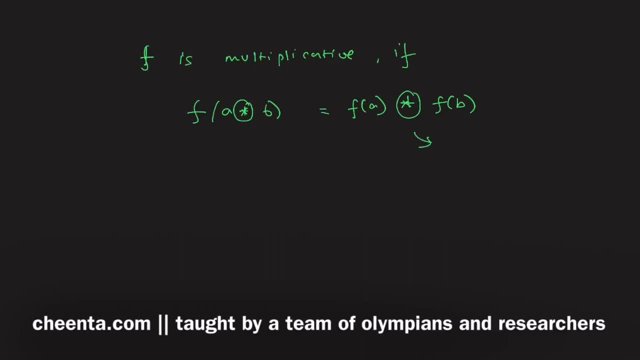 any operation that we are interested in, So operation. So, for example, star could be multiplication F a times b. we may want it to be fA times fB. Star could be addition, depending on the context. So f of A plus B, we may want it to be fA plus fB. Star may be something else. 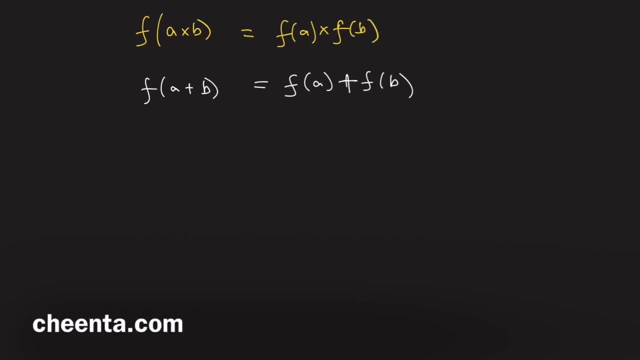 So, whatever it is, the context will tell you what star is. One example of a multiplicative function is the Euler's torsion function. We discuss it in our number theory module as well as in group theory module. Euler's torsion function counts the number of numbers, the number of numbers. 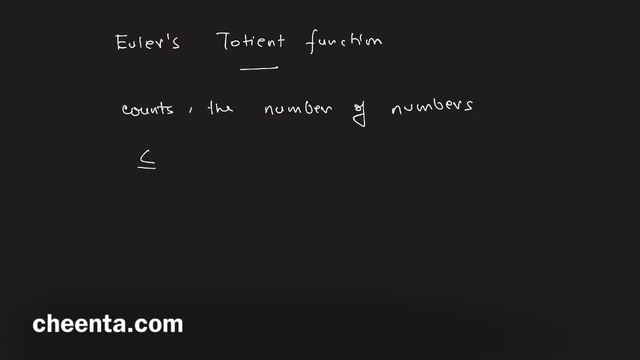 less than the number of numbers. Euler's torsion function counts the number of numbers less than or equal to n, and which has hcf 1 with n. So if A is the number, the hcf of the number with n is 1.. 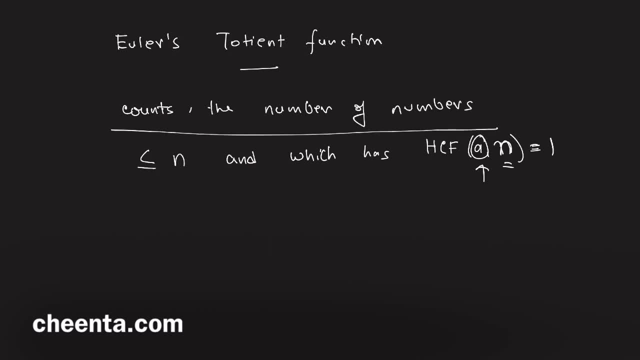 We count all such numbers. That's what the function Euler's torsion function. that's what the Euler's torsion function does. That's what the Euler's torsion function does. I'll give you an example. Suppose 8 is a number. 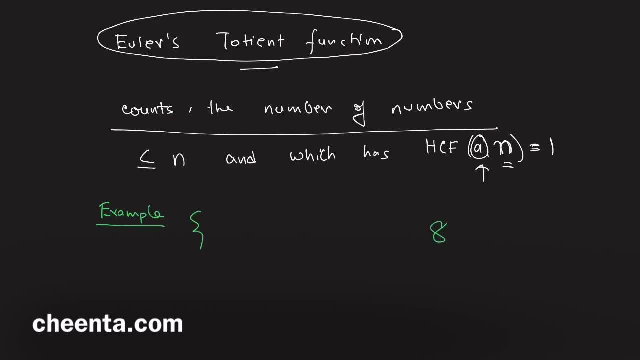 Look at all numbers less than or equal to 8, which has hcf 1 with 8.. Those numbers are 1,, 3,, 5 and 7.. For example, hcf of 1 and 8 is 1.. hcf of 3 and 8 is 1.. hcf of 5 and 8 is 1.. hcf of 6 and 8 is 1.. hcf of 7 and 8 is 1.. hcf of 8 and 8 is 1.. 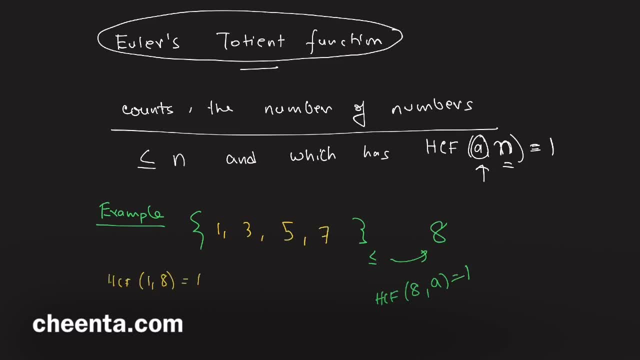 hcf of 7 and 8 is 1.. hcf of 8 and 8 is 1.. hcf of 8 and 8 is 1.. hcf of 9 and 9 is 1.. hcf of 10 and 10 is 1.. 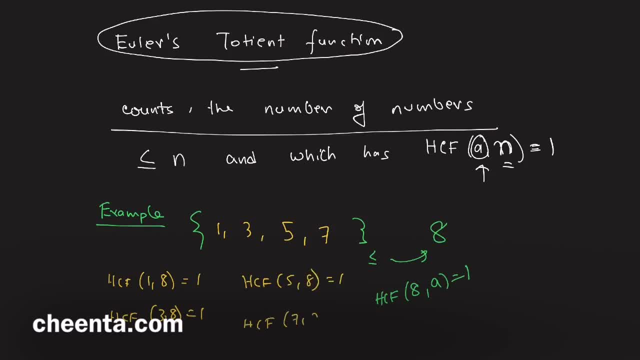 hcf and 12 and 12 is 1. hcf and 13 is equal to 1. hcf of 12 and 13 is 1. hcf and 14 is equal to 1. hcf and 15 is equal to 10 and 16 is 1.. 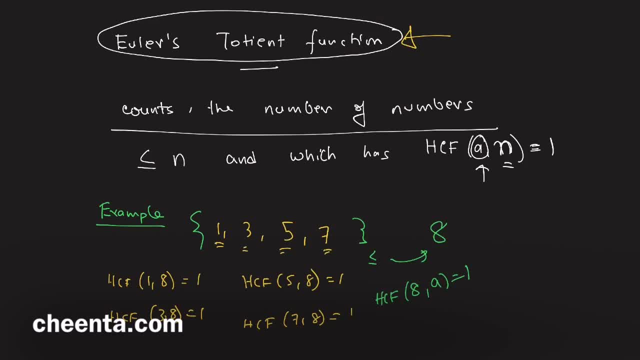 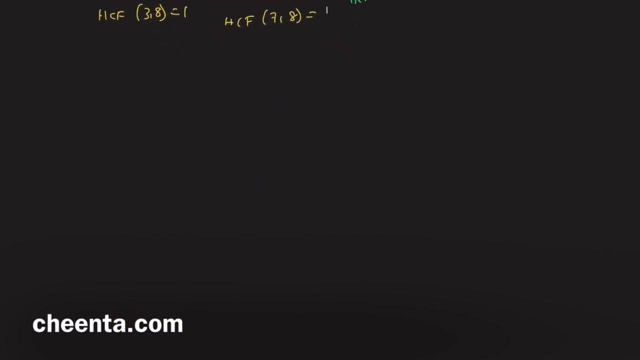 And 13.. And 13 and 13 is equal to 5,, 5,, 3,, four such numbers, which has hcf1 with 8.. Let me give you one more example to make this idea absolutely clear. What is phi of 15?? So take 15.. Let's find out all numbers less than equal to. 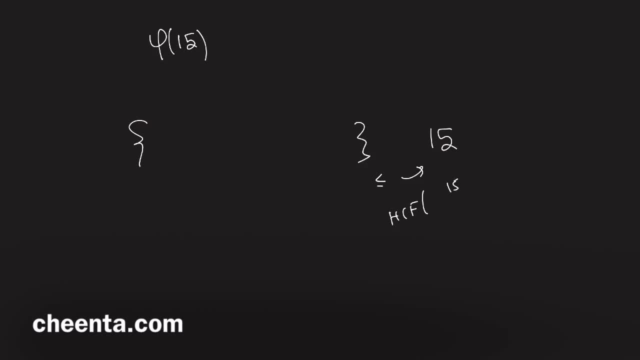 15, which has gcd1 with 15.. So those numbers are 1,, 2,, 4,, 7,, 8,, 11,, 13 and 14.. So these are the numbers. So hcf of each of these numbers is with 15 is 1.. hcf of 1 with 15 is 1.. hcf of 2 with 15: 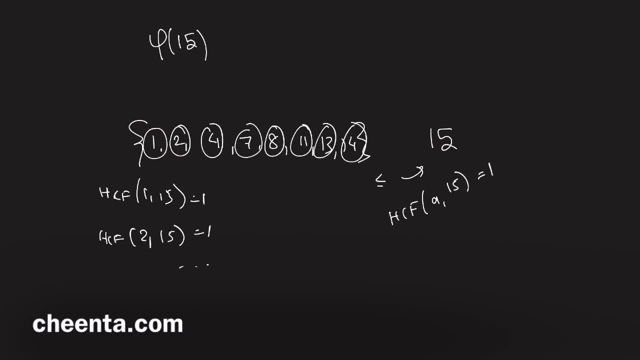 is 1 and so on. So what is phi of 15?? It will count the number of elements in this set, and that will be: phi of 15 is 8.. All right, So what is so beautiful about this function? 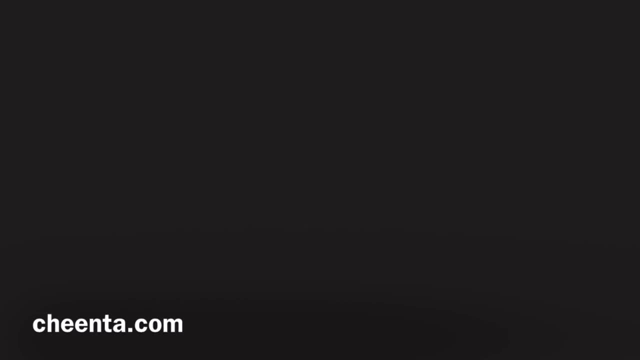 Well, this function is multiplicative. Phi function is multiplicative. Why So? for example, if I take two numbers, a and b, whose hcf is 1, then phi of a times b is equal to phi a times phi b. 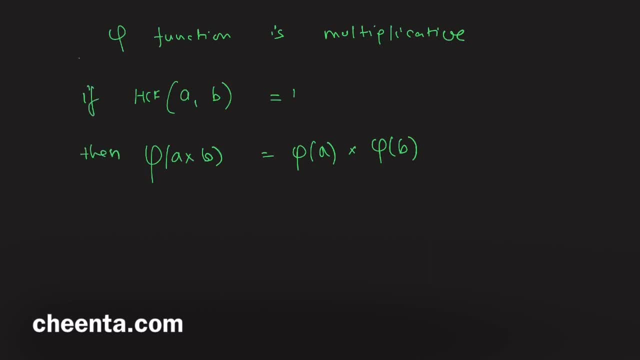 If, then So this is a theorem. One needs to prove this. This is not automatic. You need to prove this, So this will be posted in our internal video: How to prove this and how to solve more difficult problems using this property. 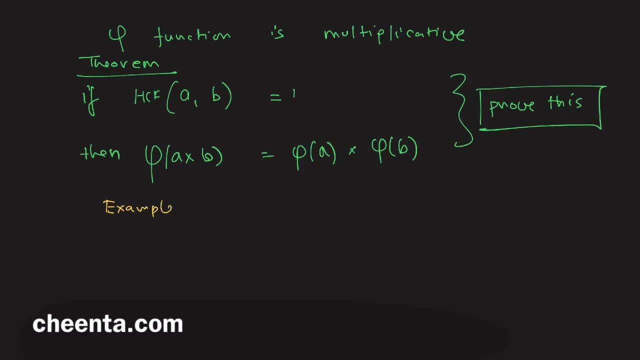 Well, let me give you an example. So, for example, hcf of 2 and 3, or maybe 3 and 4, is 1.. What is phi of 3?? So, if you look at the numbers which are less than equal to 3 and whose hcf with, 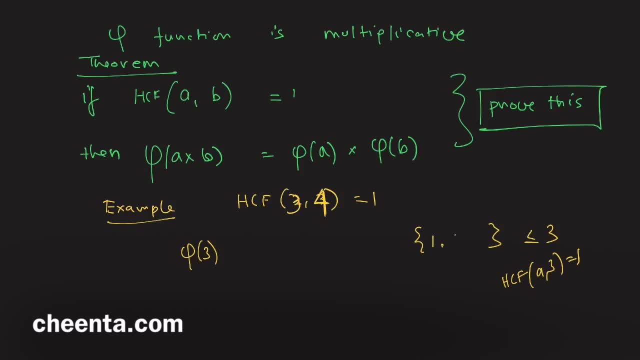 3 is 1.. Those are 1 and 2.. So phi of 3 is 2, phi of 4- you can check- is 2 as well, because numbers which are less than equal to 4 and hcf with 4 is 1. Those numbers are 1 and 3.. So there are two numbers again. 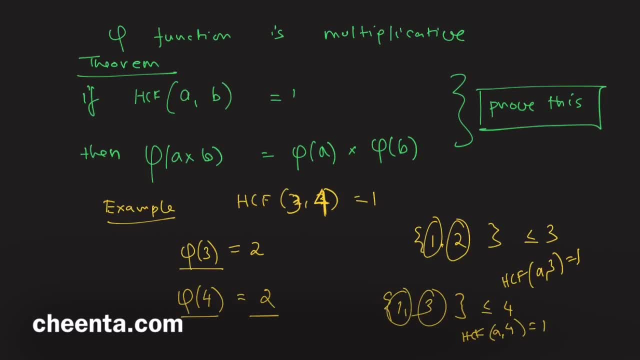 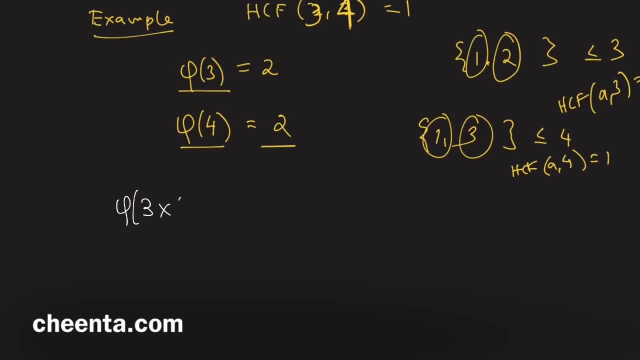 So phi of 4 is 2.. Now let us figure out. what is this multiplicative business all about? So here we have phi2 plus 3.. So if we look at our originalat vowels, what we have written down is that phi of 3 times 4 is equal to five of three times phi of four. This is the claim. We do not know this yet. We know phi of three, and that is 2.. We know for your four, that is also 2.. So two times two is 4.. We expect phi of three times forward his five of twelve to be, for we want to know if phi of three of twelve is equal to 4.. We are not sure. 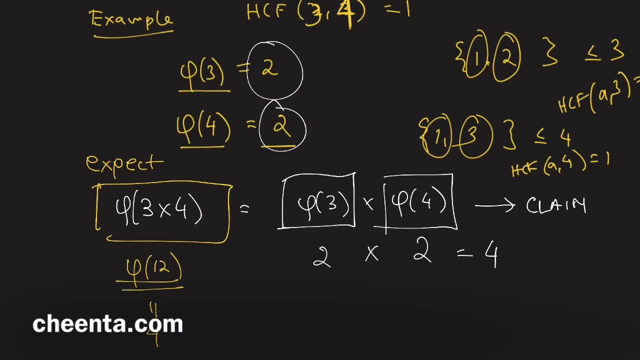 So let us predict. it's their future. Although we have known this success story, we are going to compare them as a way to dislike이스. so this to happen. let's check if that happens. so look at 12. let's find all numbers which are less. 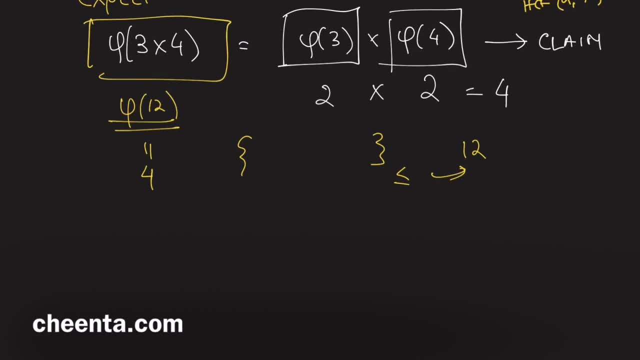 than equal to 12, whose hcf with 12 is 1. so those numbers are 1. 2, 3 will not work, 2 will not work, 3 will not work, 4 will not work, 5, 6 will not work, 7, 8 will not work, 9 will not work, 10 will not work. 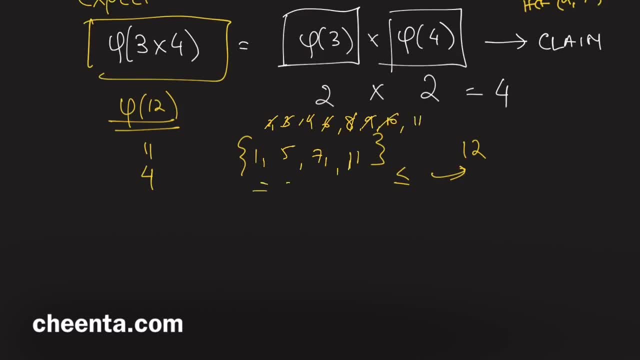 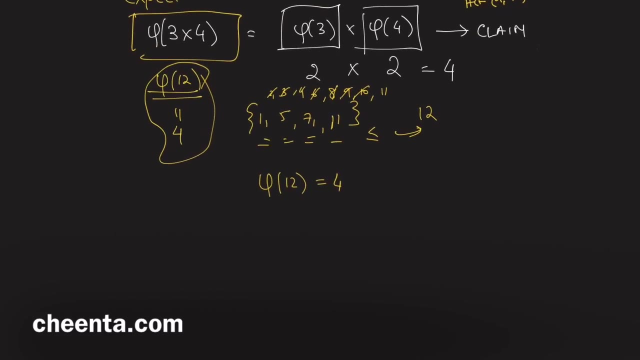 11, so four numbers. so 5 of 12 is 4, as expected, right? this is the essence of multiplicative property. why is the torsion function multiplicative? why is the torsion function multiplicative? we will discuss this in our internal video and in our class lectures.